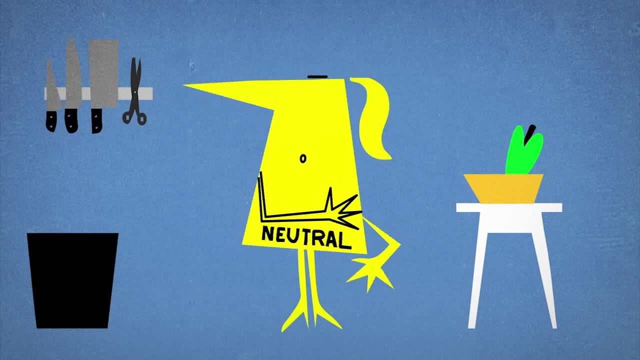 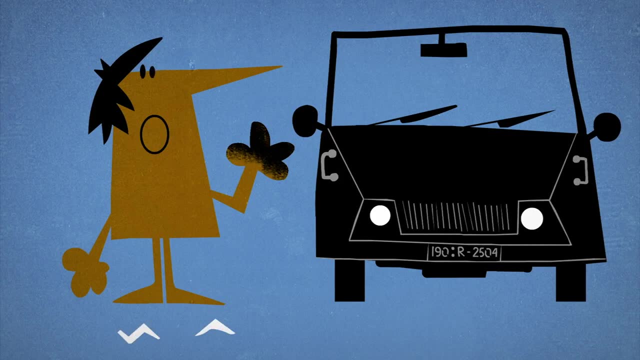 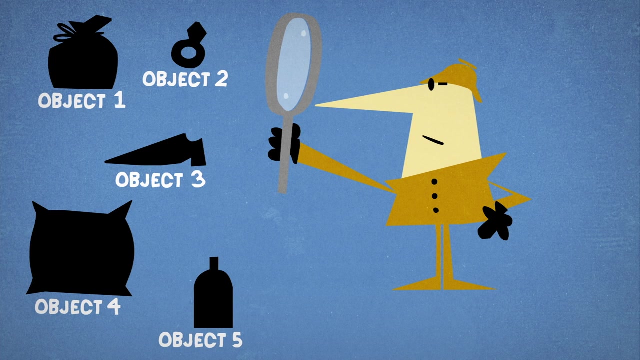 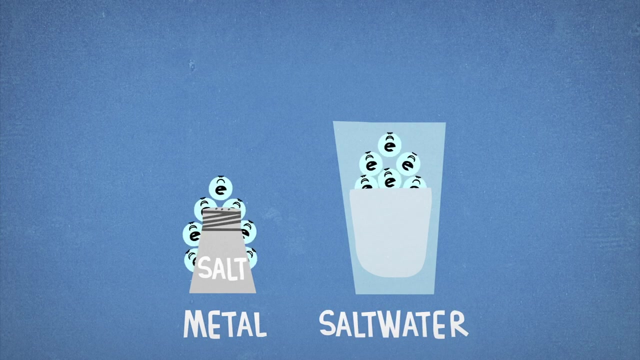 charged object or jumping onto the positively charged one in an attempt to restore the neutral charge equilibrium. And this quick movement of electrons, called static discharge, is what we recognize as that sudden spark. This process doesn't happen with just any objects, Otherwise you'd be getting zapped all the time. Conductors like metals and saltwater. 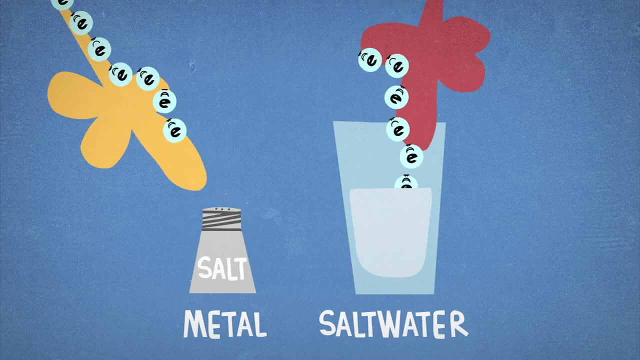 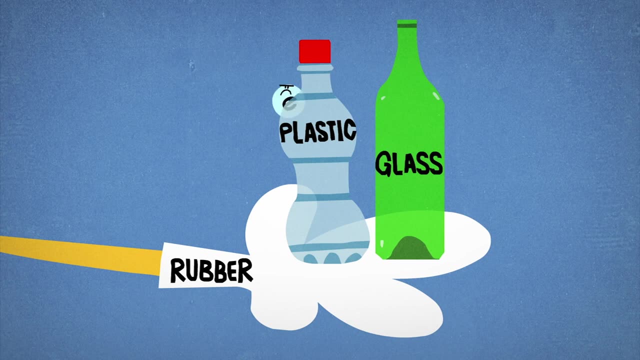 tend to have loosely bound outer electrons, and the electrons tend to get stuck in the particles, which can easily flow between molecules. On the other hand, insulators like plastics, rubber and glass have tightly bound electrons that won't readily jump to other. 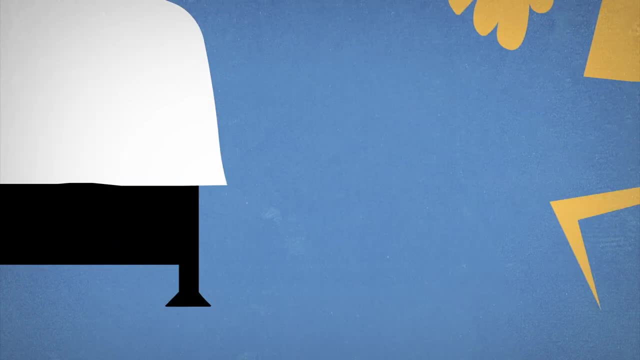 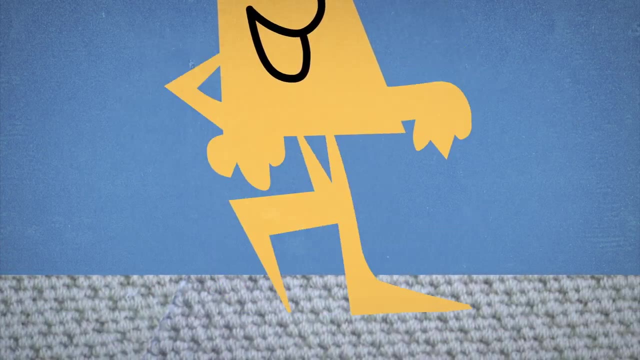 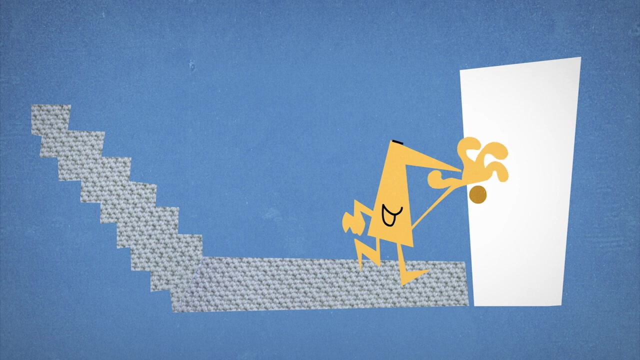 atoms. Static buildup is most likely to occur when one of the materials involved is an insulator. When you walk across a rug, electrons from your body will rub off onto it, while the rug's insulating wool will resist losing its own electrons, Although your body and the 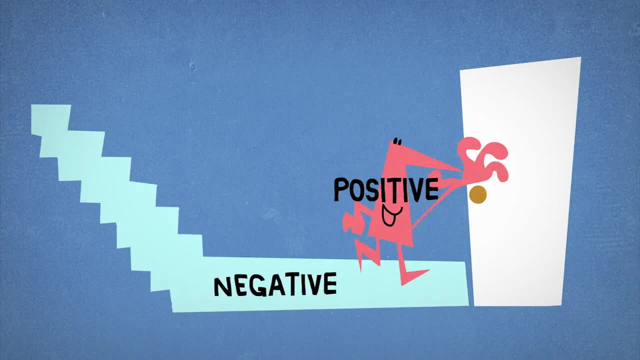 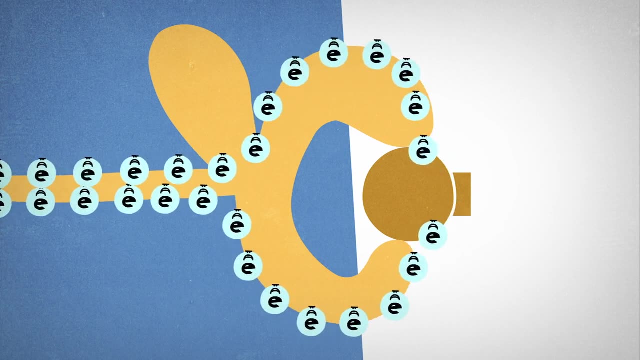 rug. together are insulated. electrons from your body will not, When the two are still electrically neutral. there is now a charge polarization between the two And when you reach to touch the doorknob, zap the metal doorknob's loosely bound electrons. 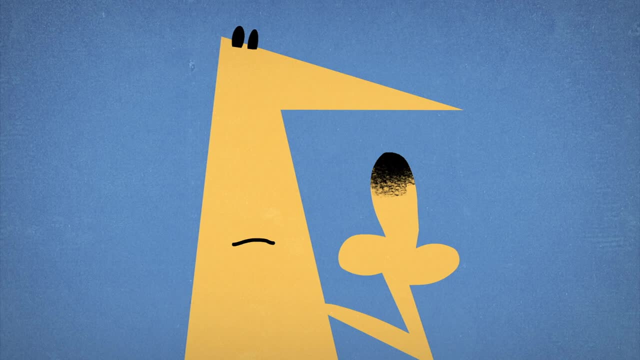 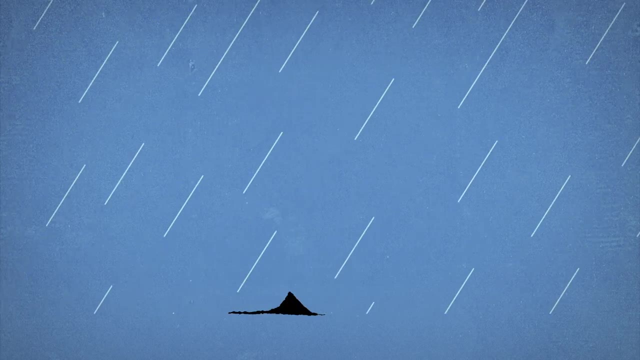 hop to your hand to replace the electrons your body has lost. When it happens in your bedroom, it's a minor nuisance, But in the great outdoors, static electricity can be a terrifying destructive force of nature. In certain conditions, charge separation will. 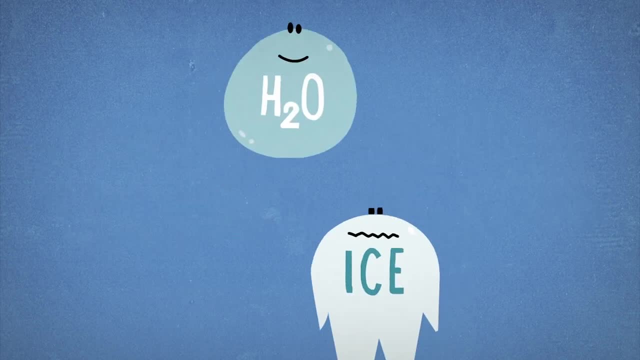 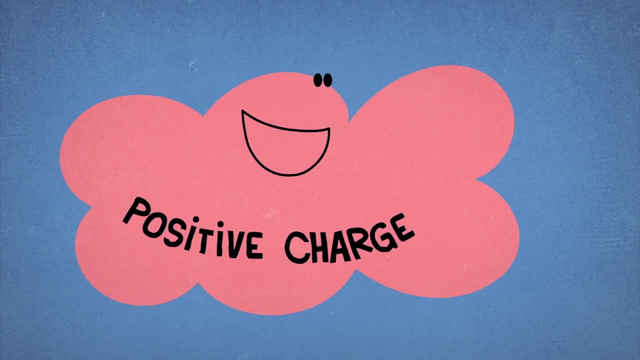 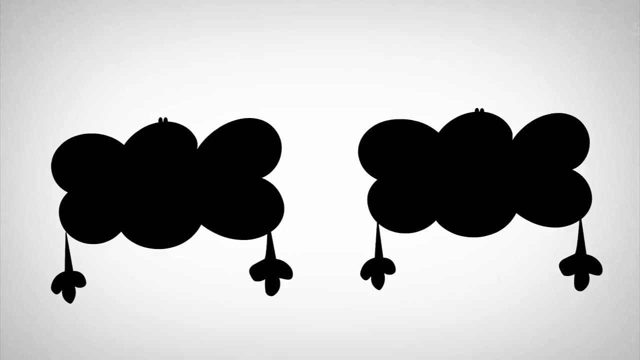 occur in clouds. We don't know exactly how this happens. It may have to do with the circulation of water droplets and ice particles within them. Regardless, the charge imbalance is neutralized by being released towards another body, such as a building, the earth or another cloud, in a giant spark that we know as lightning. 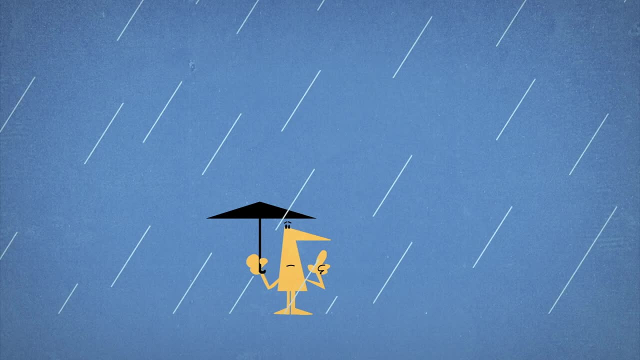 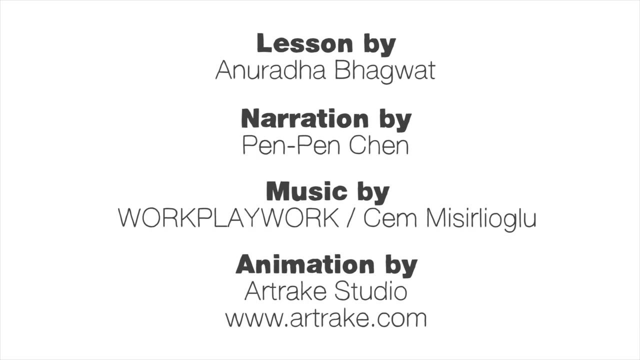 And just as your fingers can be zapped over and over in the same spot, you better believe that lightning can strike the same place more than once. Thanks for watching and I'll see you in the next video.